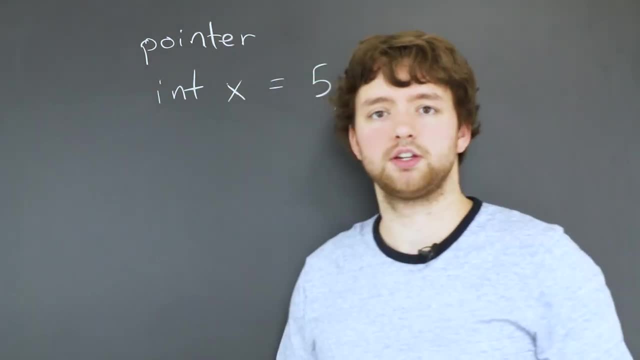 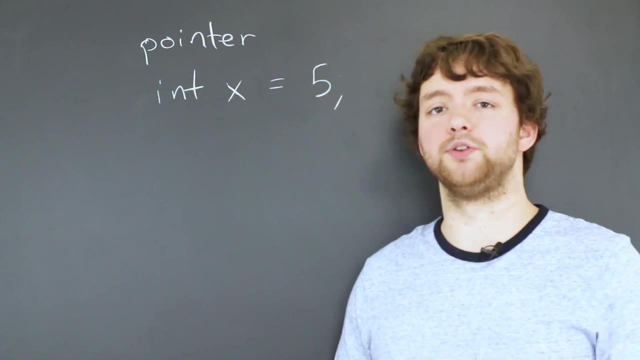 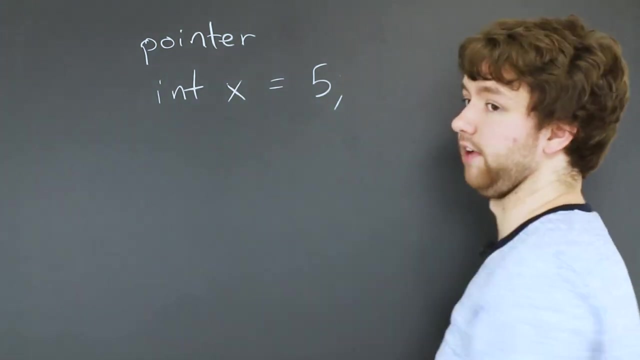 assigned some value. now, when we do this, inside of our computer there's an area called of memory, area of memory. another name for memory is ram. so inside of our memory there is a spot holding the value of x. so if you want to think about it that way, just there's a cell in our memory with the 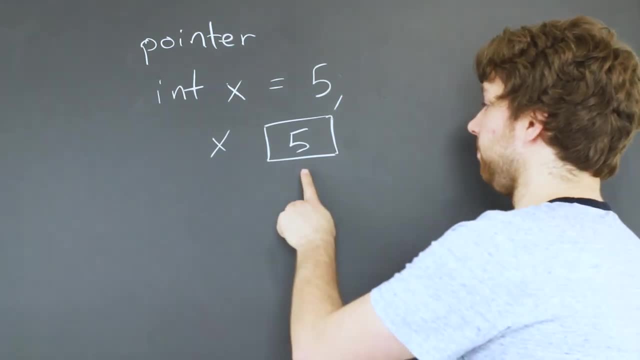 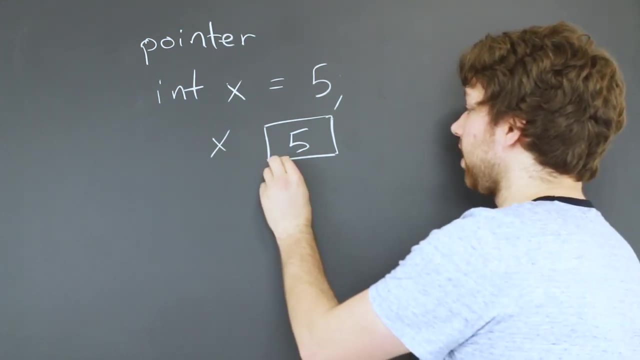 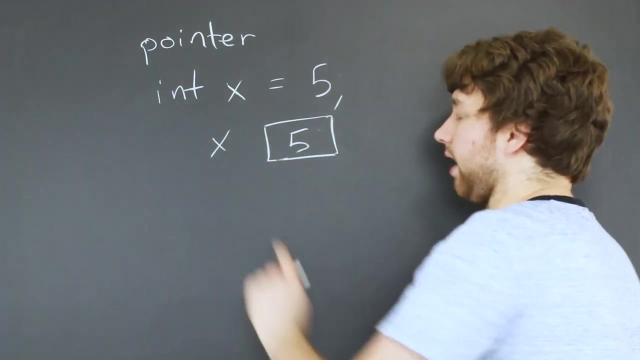 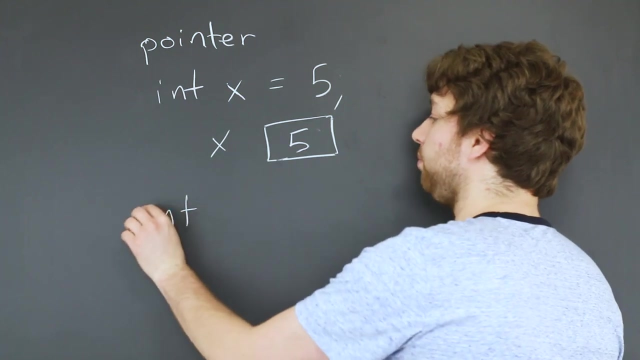 value five. now, a pointer is a way to point to this location of memory. so we can actually, uh, basically change the value of this memory or refer, reference it, but not using the variable x. we're referencing it indirectly through a pointer. the way you create a pointer is you say what type you want to point to. so we're going to point to an. 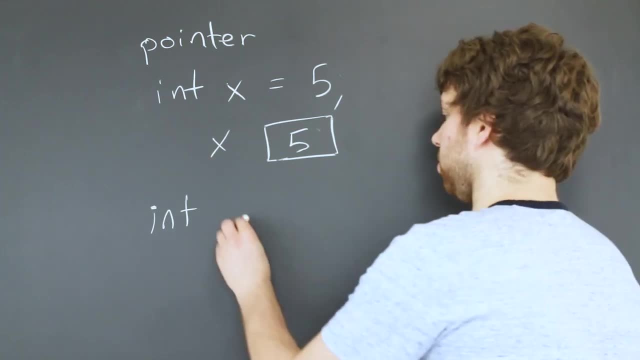 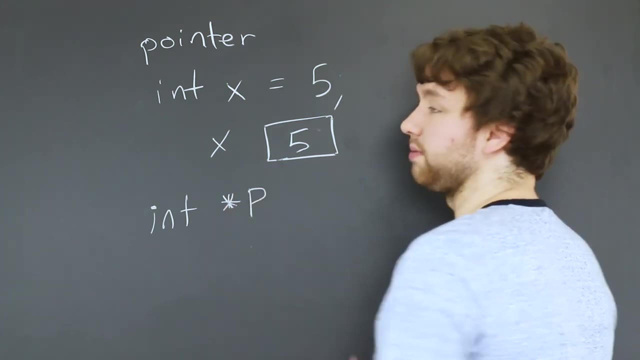 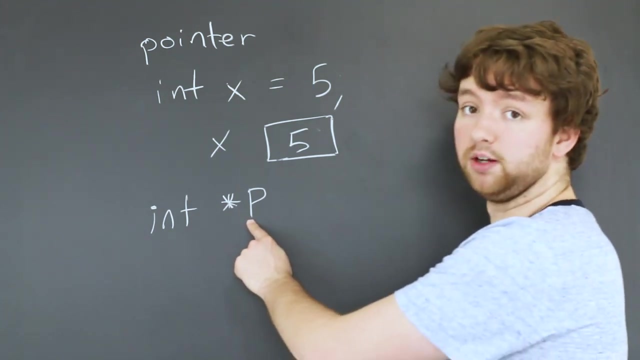 int and then you give it a name. so, um, what we're going to say, pound signed p- you have to use the pound sign and that is to indicate that it's a pointer. typically that's attached to the name of the variable here. and then what you can say is: you can set it equal to a value, just like we do this. 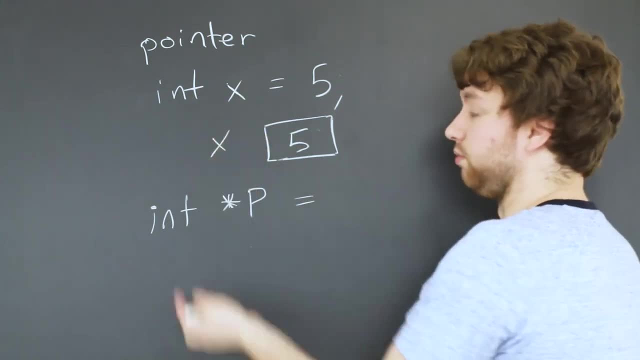 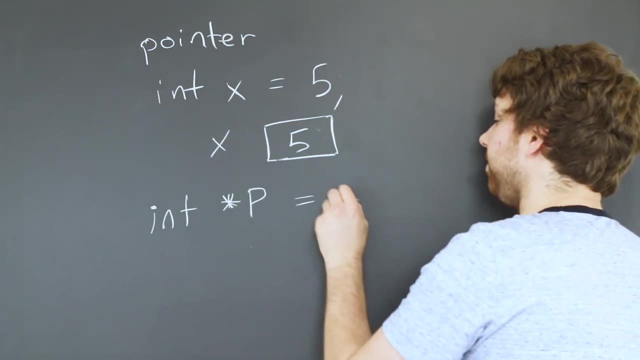 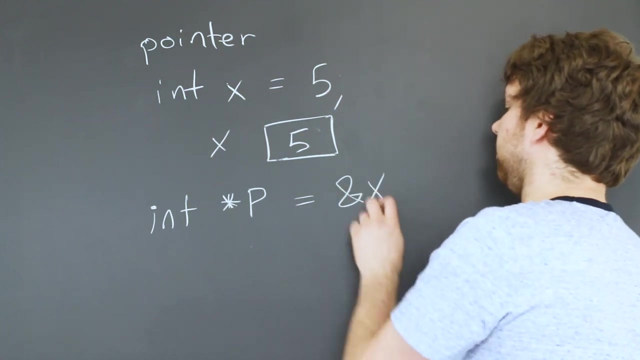 this is. this is a an integer variable x. well, here this is an integer pointer p. then what we do is we can use the address of operator, which we talked about in earlier videos, but that's going to get the address of a variable in memory x, and what this is going to do is it's going to create a variable p. 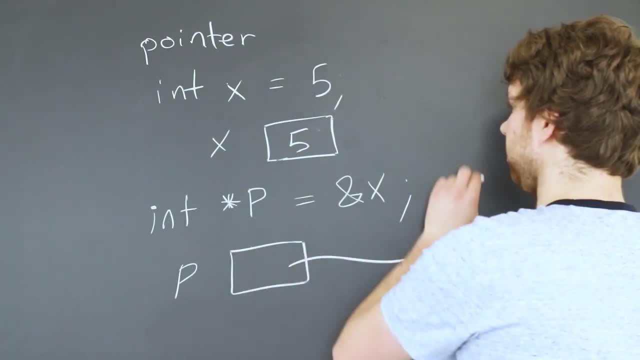 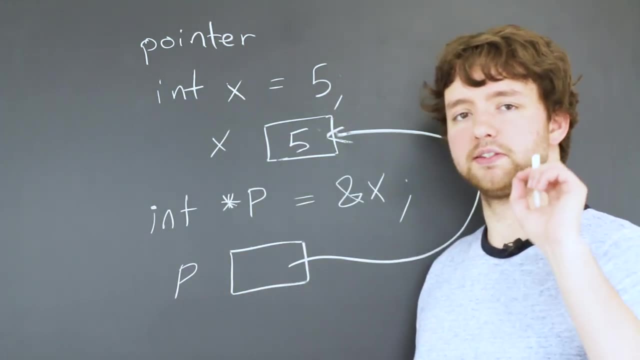 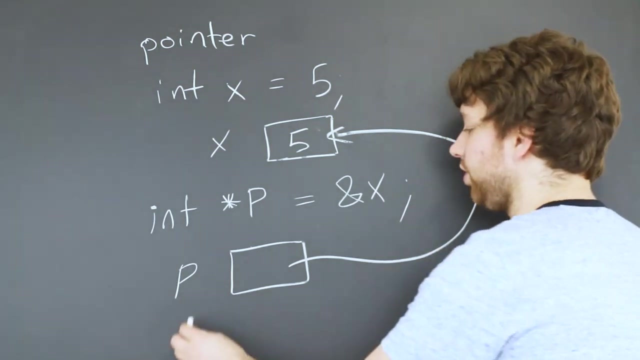 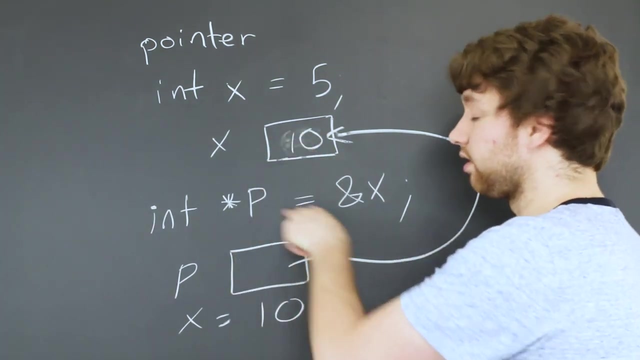 and it's going to point to five. so it's kind of like a variable equal to five, but not quite. it's the, the address of the variable equal to five. so that means if we change x to 10, well, that means we replaced this value with 10.. thus the the pointer now points to 10.. same thing we can actually change. 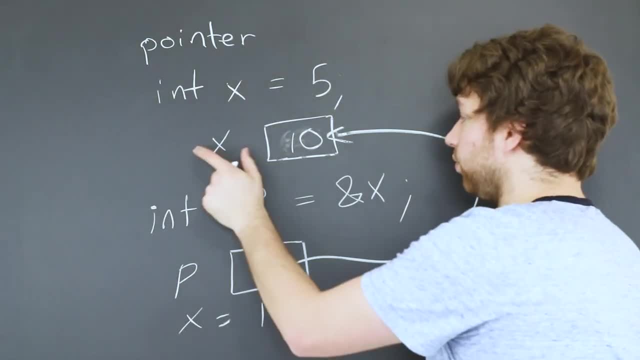 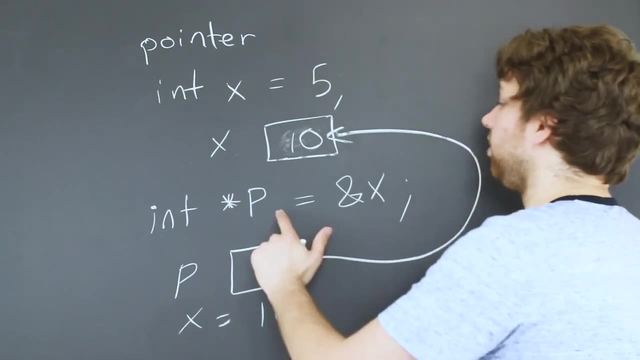 change the value through the pointer. So essentially now we have the original variable containing the value 10 and we made another variable to to point to the same data through a pointer pointing to the value 10.. So it's kind of like having two variables and they can both be. 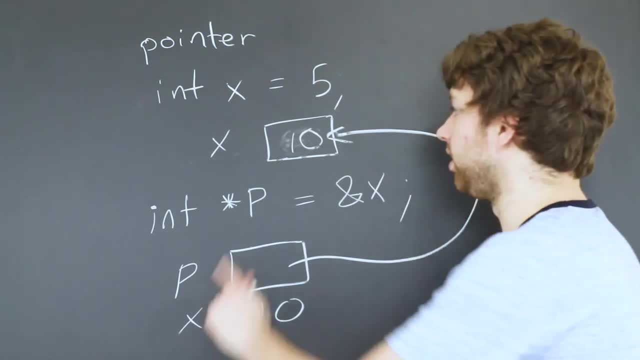 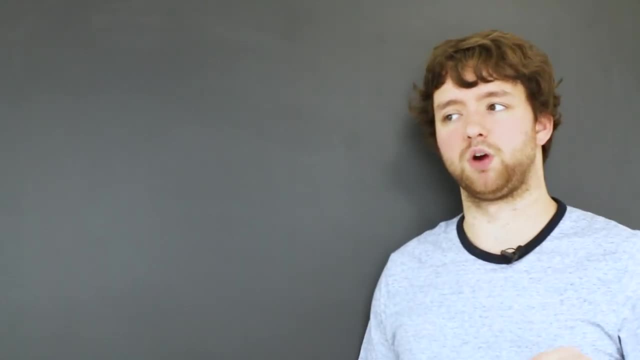 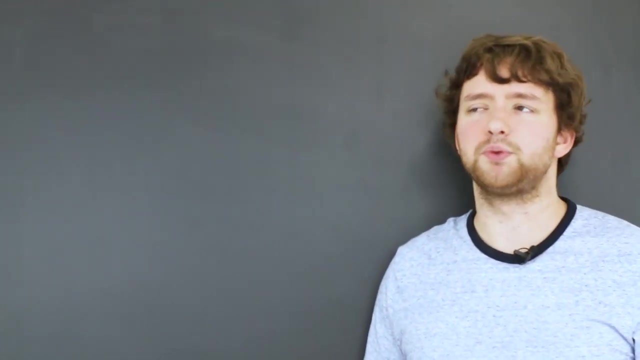 used to reference the same data, One directly and one indirectly- through a pointer. So pointers can be a little bit confusing at first, because it's kind of like one of those things where it's hard to see the benefit of them until you use them a bunch, and it's kind of like when you're a kid. 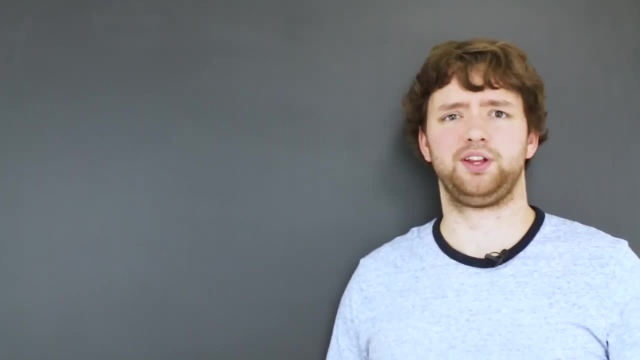 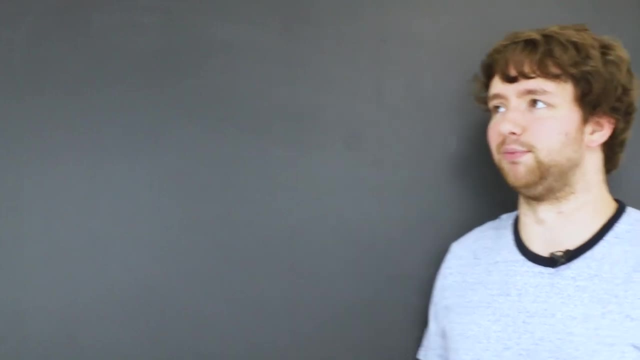 and you're starting to learn multiplication, You're like: what am I ever going to do with this in life? But as you're older, you start to understand those things. Maybe that was a terrible example. It's just something you have to practice. and then you're like: oh, I see how this is beneficial. but 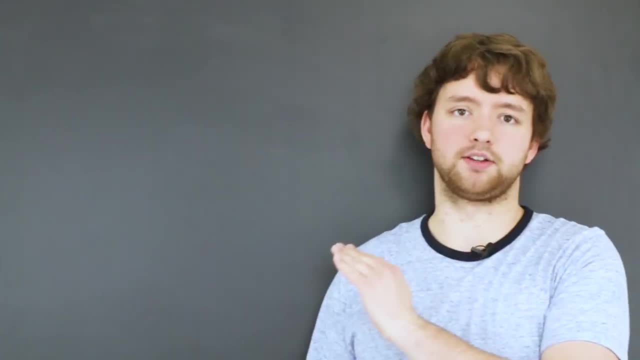 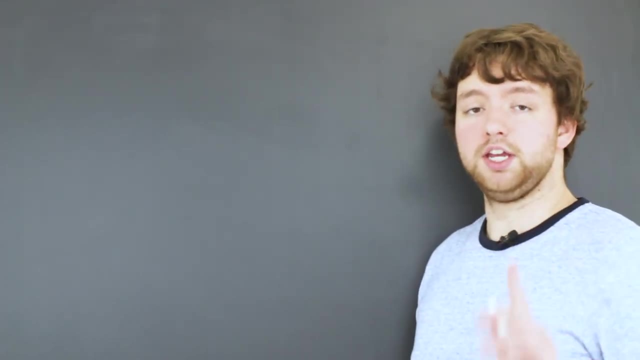 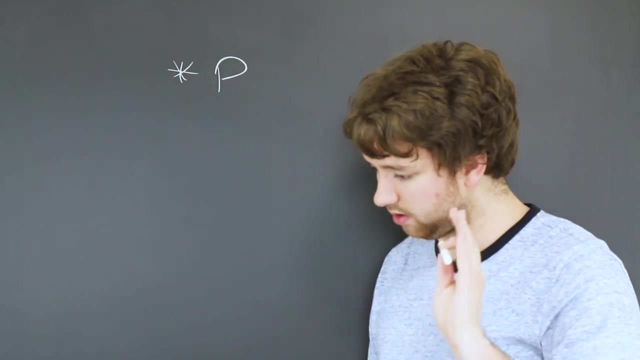 for now, just learn the fundamentals and understand these concepts, and I promise you it'll be valuable later. So the next thing you need to know is what's known as the indirection operator, and it looks like the asterisk, So this is confusing. This is what I don't like, but we just have to deal with it. When we declared the variable p, 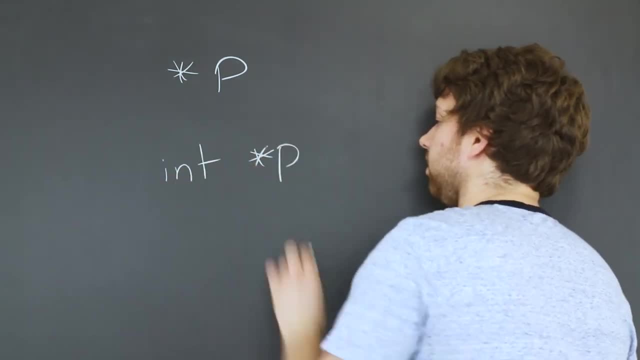 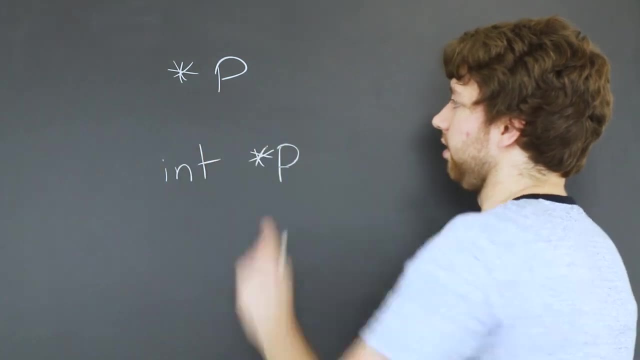 we did it like so and this, this asterisk here says: this is a pointer. This is different than the asterisk here, which is the indirection operator. I hate that, but we just got to deal with it. So when we declare the indirection operator, we just have to deal with it. So when we declare 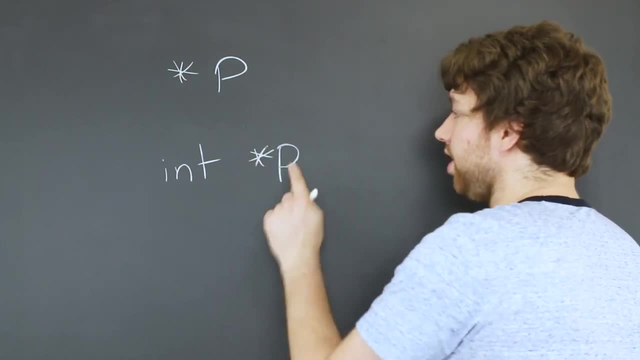 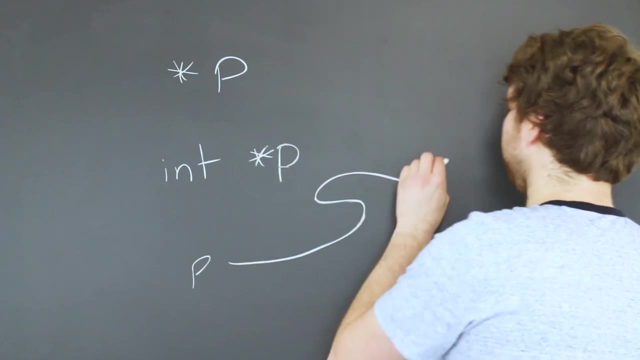 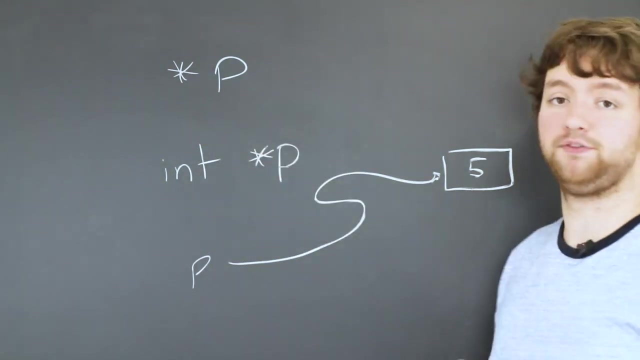 the variable we we use an asterisk Then if we want to get the value that that variable was pointing to. so p points to the value 5.. If we want to get that value, we use the indirection operator before the: the variable p. So what that means, since p was originally pointing to x. 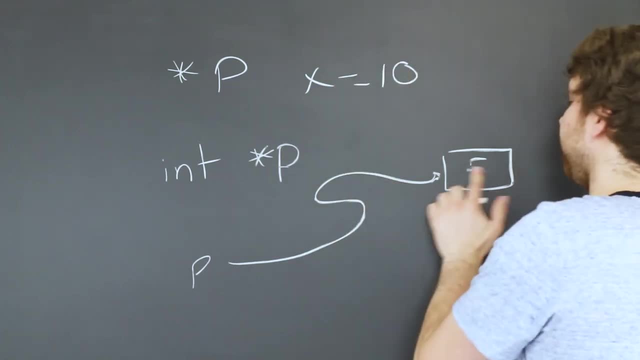 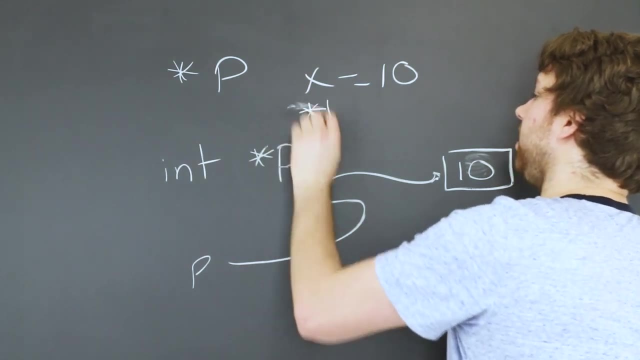 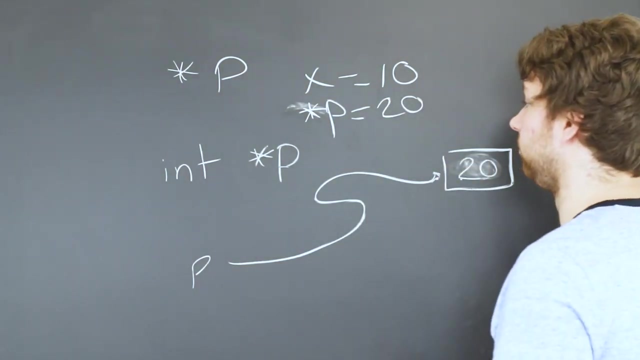 what we could do is we could say x equals 10 and change that value to 10.. Or what we could do is we could say the, the value at p is equal to 20, and that'll change the value. At this point, if you printed x, it would print 20.. So the benefit here: 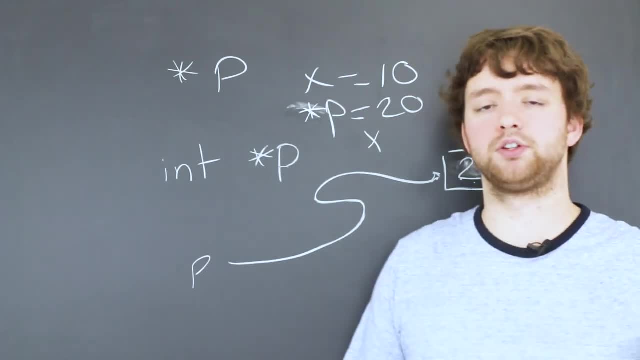 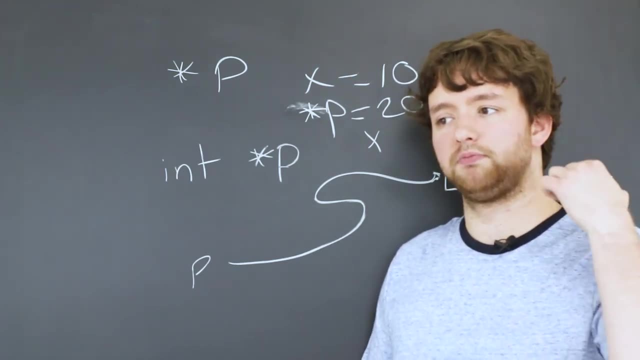 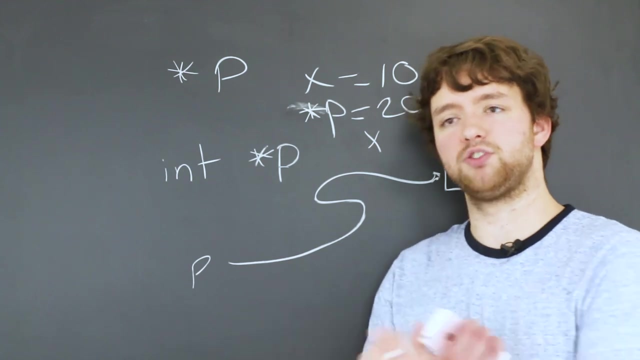 is that once we understand pointers, we can use pointers to functions and these. this will allow functions to change the values of variables, And that can be really valuable if you need to do something like a swap function. You're not able to change the value of variables unless you're